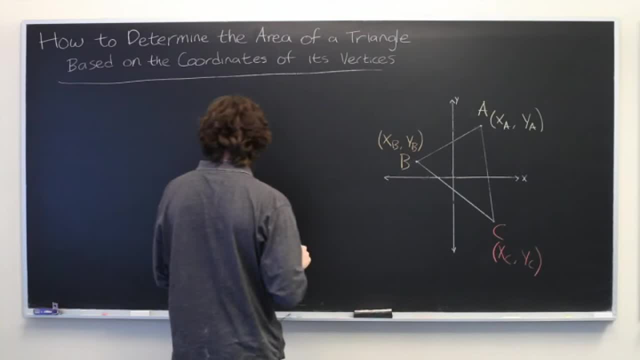 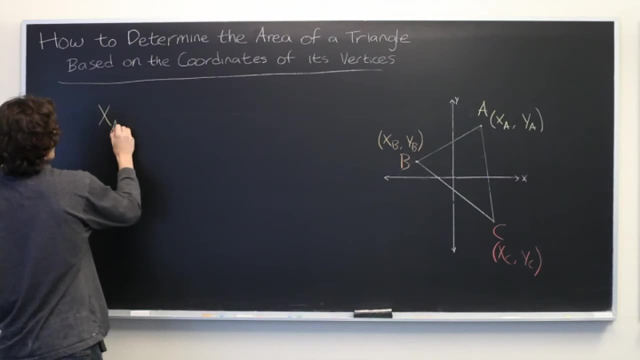 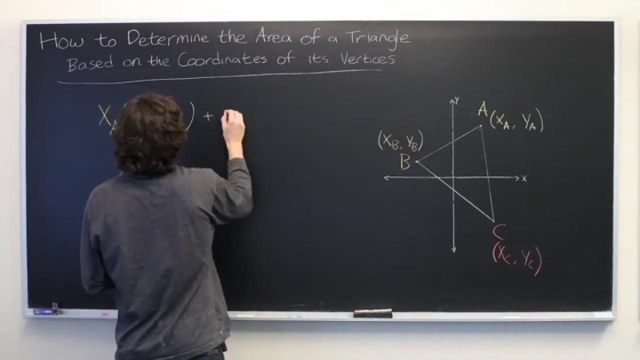 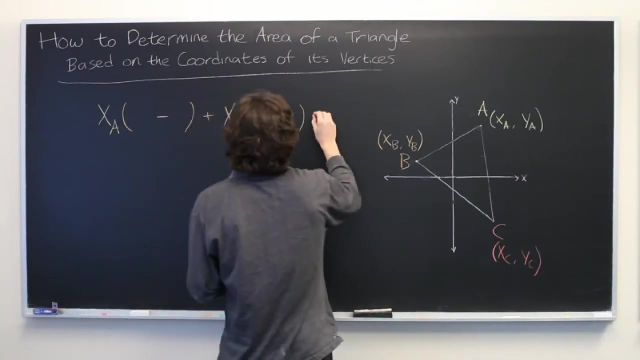 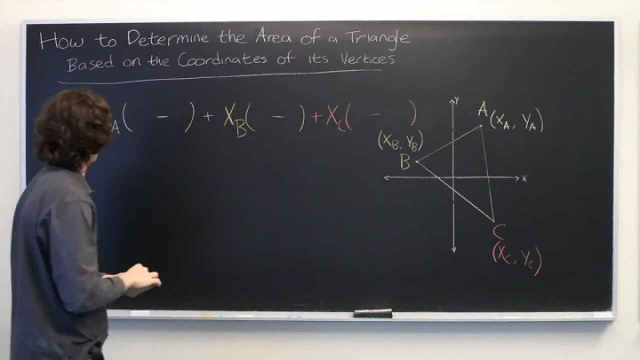 but it's not terribly difficult to calculate, So we'll set it up piece by piece. I'm going to have xa times some quantity, which we'll fill in afterwards, plus xb times some quantity, plus xc times some quantity. Okay, now let's fill in these values. So in here we 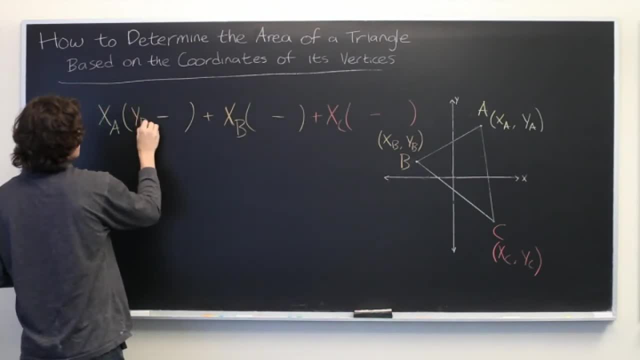 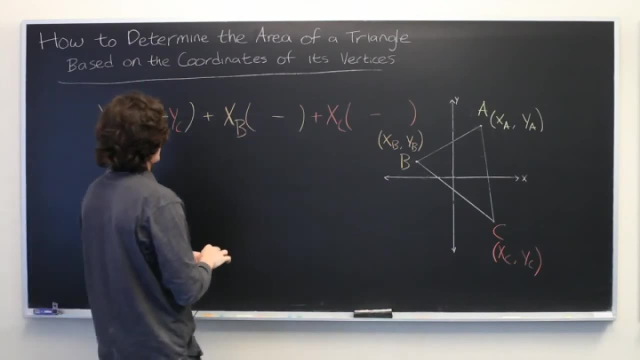 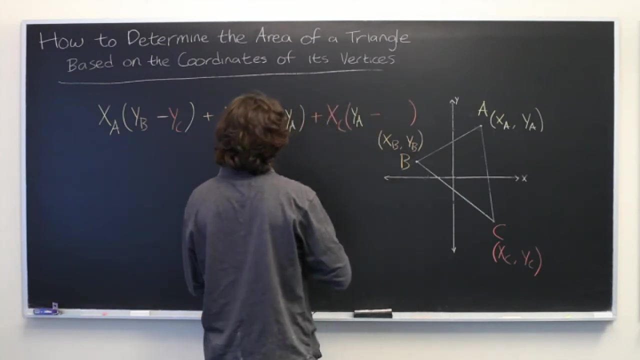 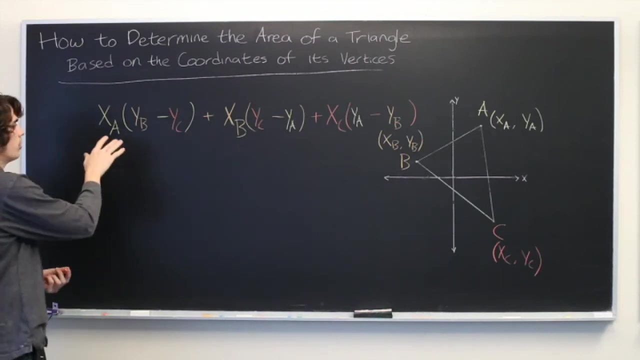 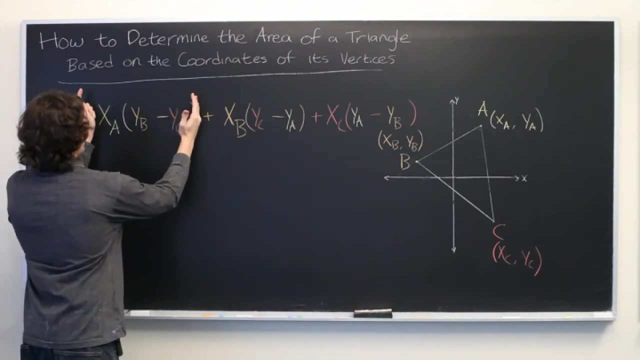 have yb minus yc. then we have yc minus ya. finally we have ya minus yb. Now it may be somewhat confusing to remember which order these letters go in, but the easiest way to remember is when you look at any one chunk. a, b and c should be in the right order: a, b, c, and here it's. 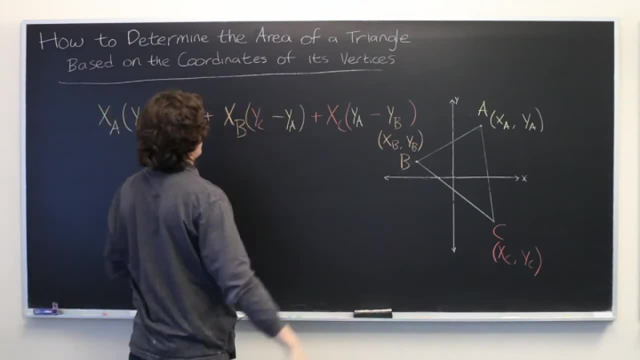 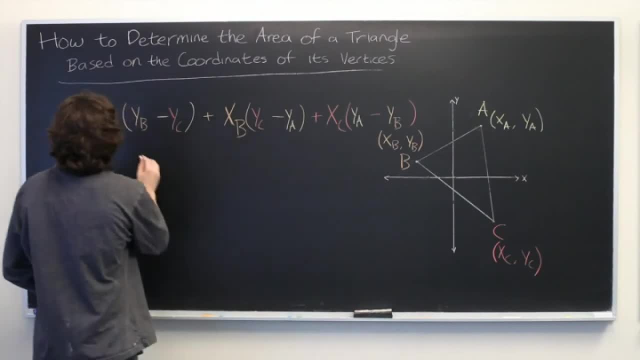 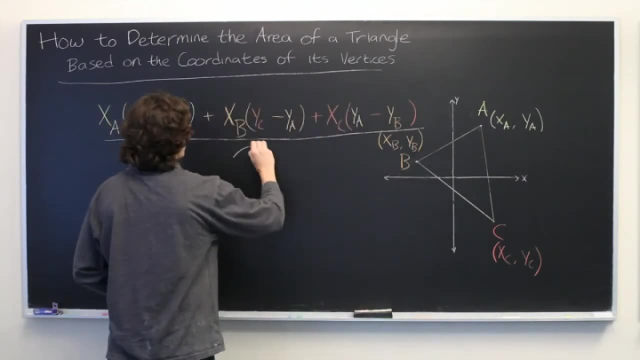 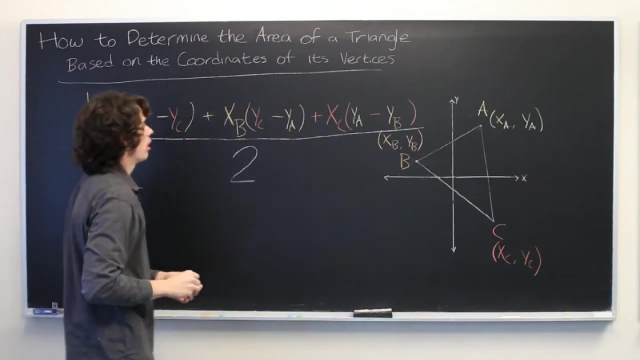 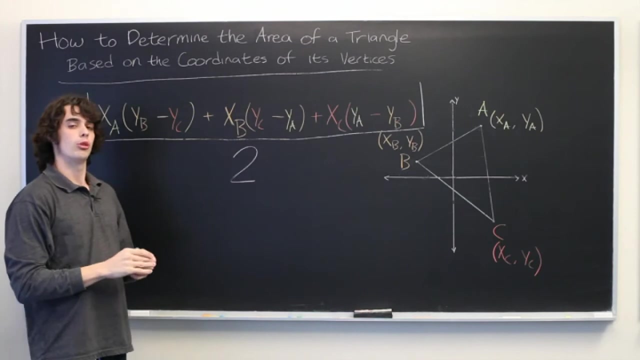 going to do is we're going to divide all of this by 2. And, finally, we're going to take the absolute value of the top part in order to ensure that we do in fact get a positive area, since it doesn't really make any sense for a triangle to have negative area A couple. 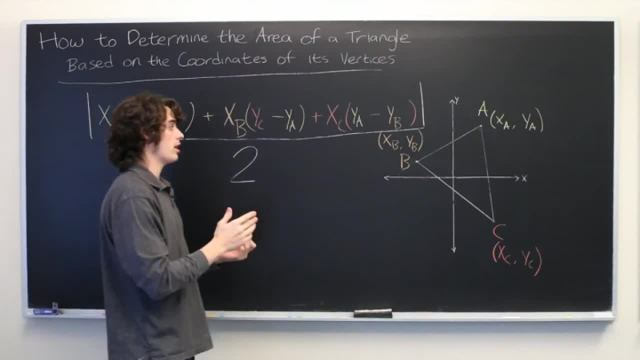 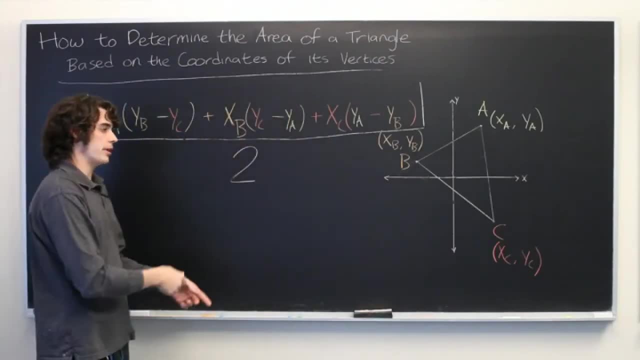 things to keep in mind about this is that this will work even if some or all of the coordinates are negative, as you can see here, And also if you compute this and find that the area is 0,. what that means is that the three points of